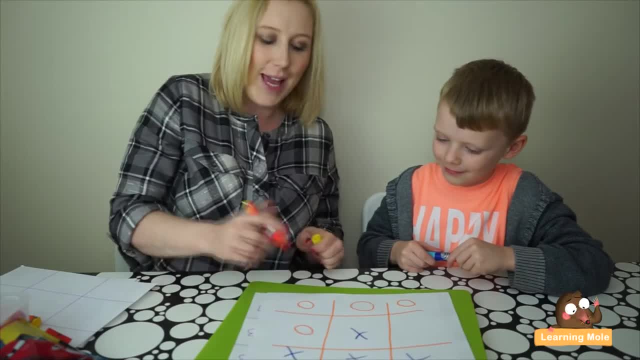 just as I thought I'd won and I was being really sneaky. Okay, so Aaron's got his three X's in a row first. Okay, so Aaron's got his three X's in a row first. Okay, so Aaron's got his three X's in a row first. 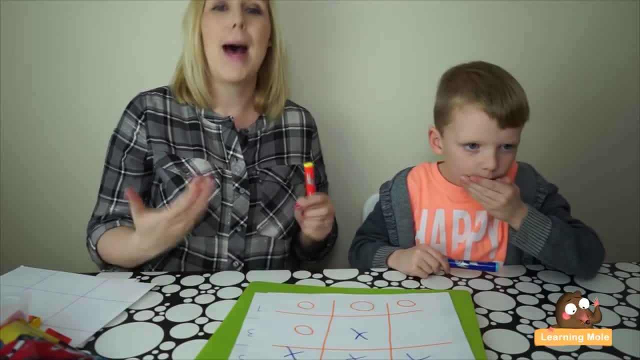 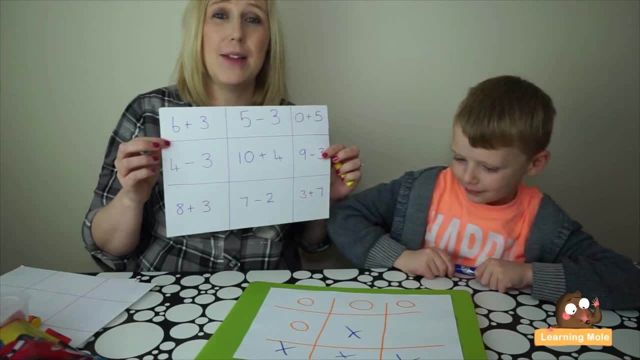 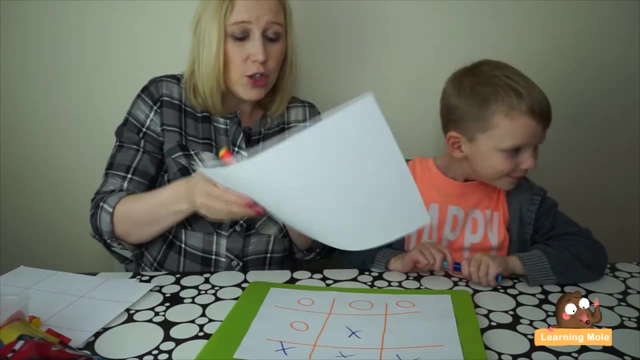 Okay, so what we want to do is take this into maths capacity now. So all I have done is I've prepared the exact same grid but with different maths calculations, and again, this is easily adapted to whatever your child's ability is actually at. So if you want to do all addition, 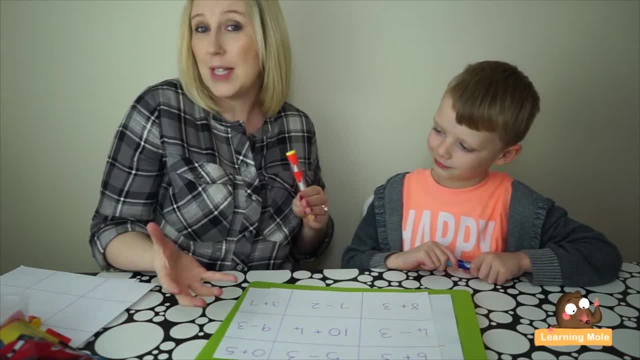 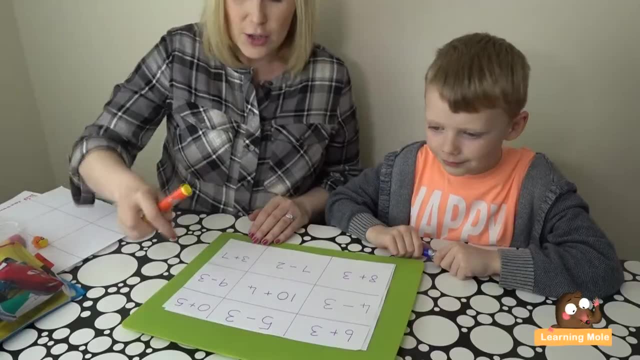 or you want to do all subtraction, or you want to focus on times tables. it's entirely up to you. You set the sums and you set what will challenge your child. So, Aaron, this time it's a wee bit more difficult. Okay, so you have to still put your X's and your O's. 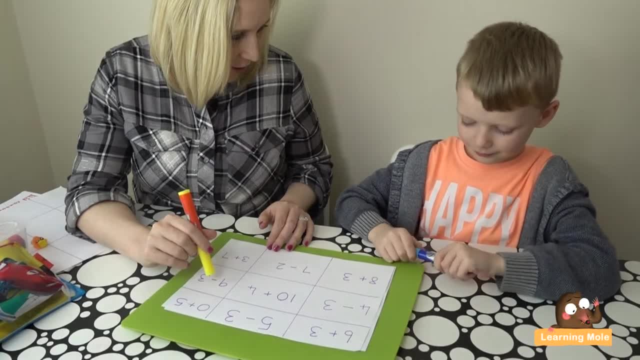 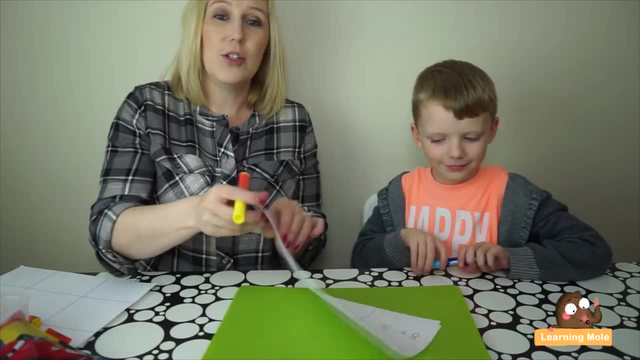 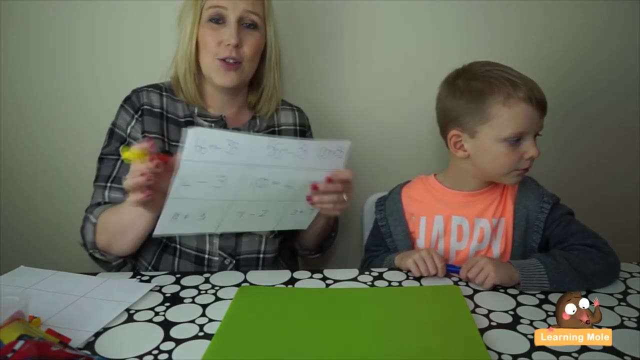 in, but you have to do a maths question first. Okay, do you think you can do it? That's the one you're going to choose first, Okay. so basically, all you're doing is you're asking your child to choose which square they want. They have to solve the question before they can put their X or their O into that. 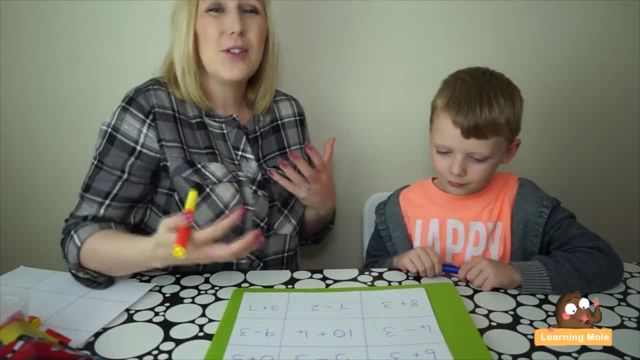 little section and again you're looking for that idea of getting three in a row, but just a really nice way of challenging your child. So, Aaron, you're going to do a maths question first. Okay, so you're challenging your child and having a little fun game and it doesn't take much time to set up. 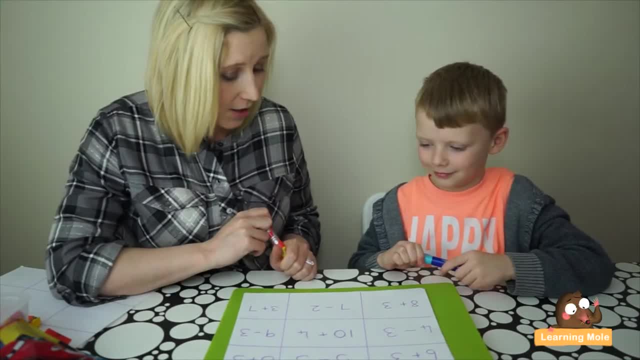 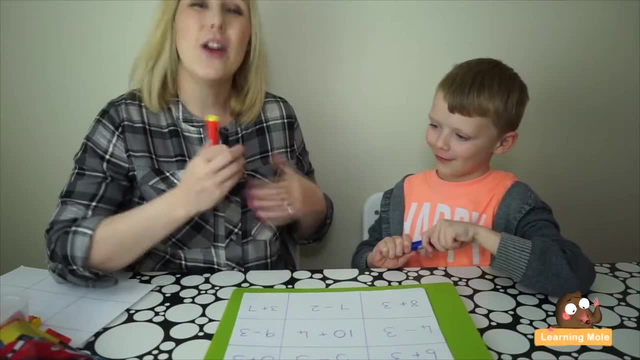 Okay. so, Aaron, where are you going to go first? Tell me which calculation are you going to try and solve first? What's that Zero plus five? Encourage your child to actually read the calculation so that they know exactly what they're doing. 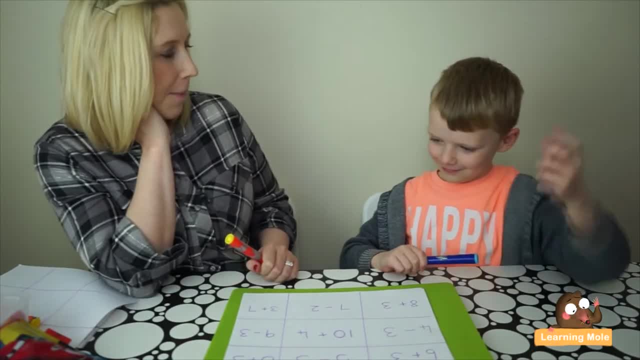 So zero plus five. So how are you going to do this in your head? Tell me: Okay, you're going to do it in your head, but how are you going to do it? What number are you going to put in your head first? 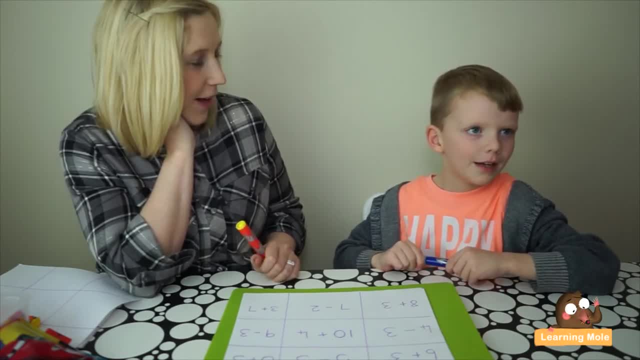 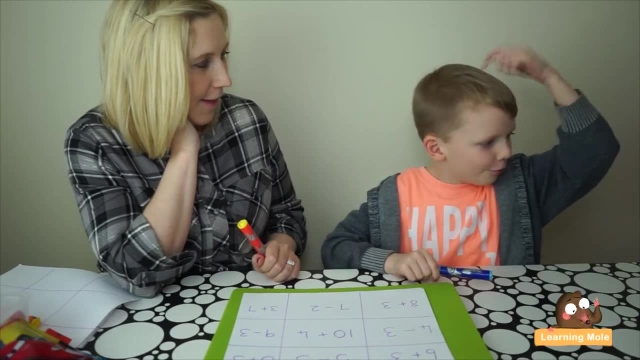 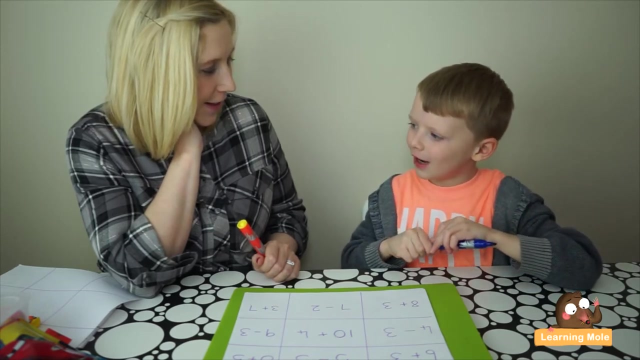 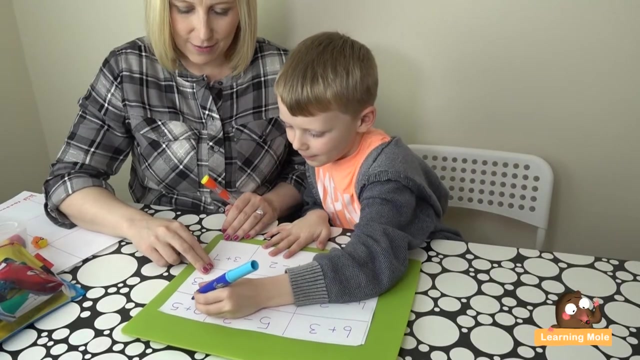 Well, five. Why are you putting five first? Because zero is nothing. Okay, Five, zero. All right, you have to tell me the answer. It's five. Five plus zero equals Five. You are correct. All right, you can put your X, put a big, nice big X right through that whole number. 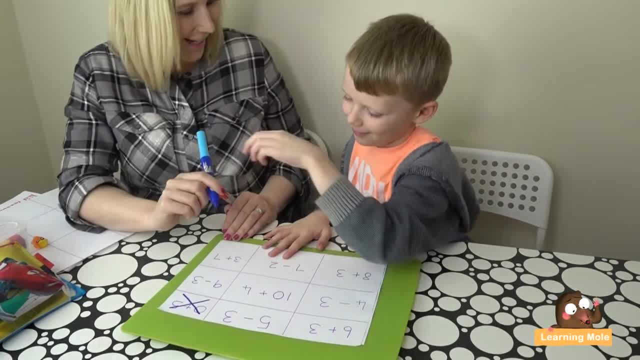 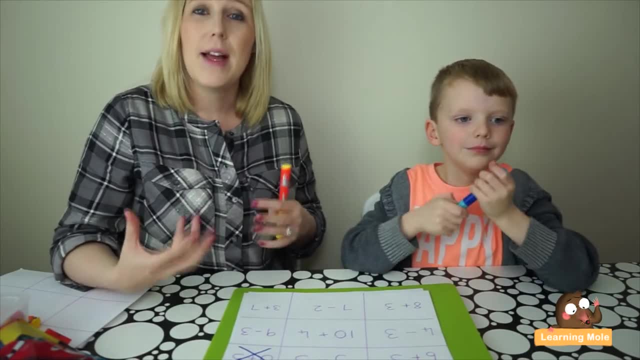 Put it right through the whole number sentence like this: Ta-da, Good boy. Okay, really encourage your child to talk about what they're doing mentally and actually start developing those ideas of putting that biggest number first, especially if it's addition, and starting to get them. 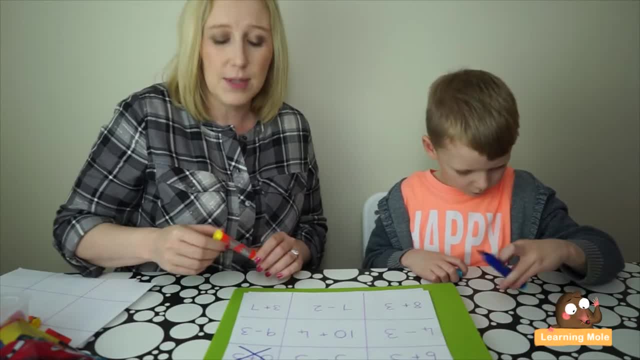 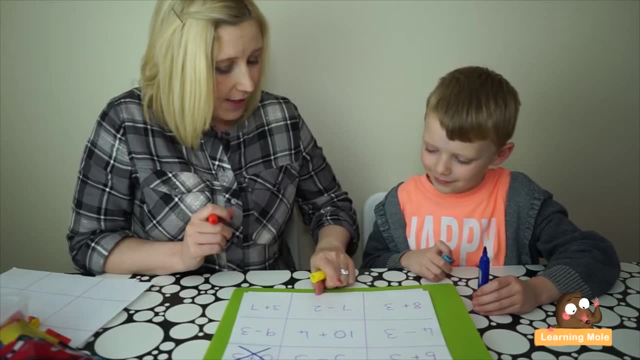 to think about how they're thinking and how they're solving those calculations. Okay, right, mummy is going to do I think mummy is going to do seven. take away two, Okay. so do you know what I'm going to do? What? 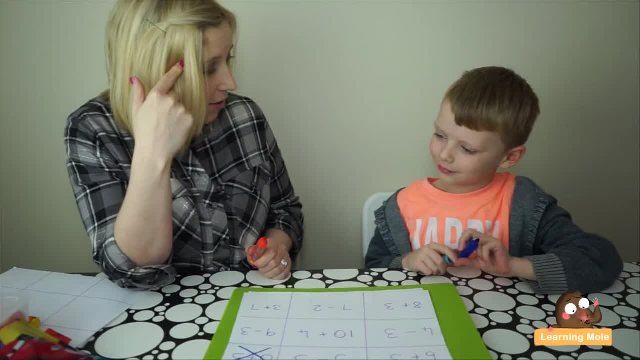 I'm going to put seven in my head, because when we're taking away the biggest number all the time, because when we're taking away the biggest number, always has to go first, doesn't it? And I'm going to count back two, but I'm going to use my fingers. 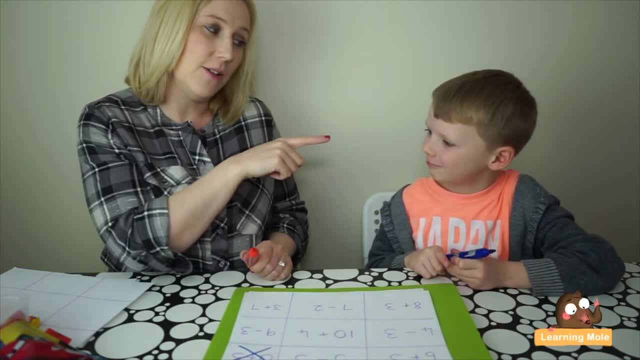 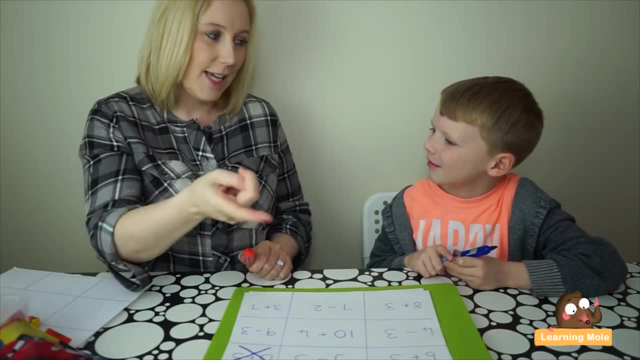 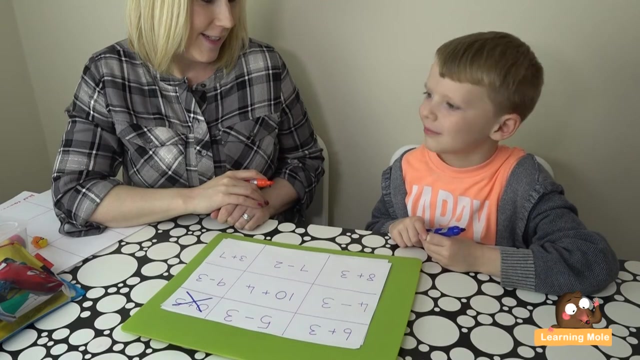 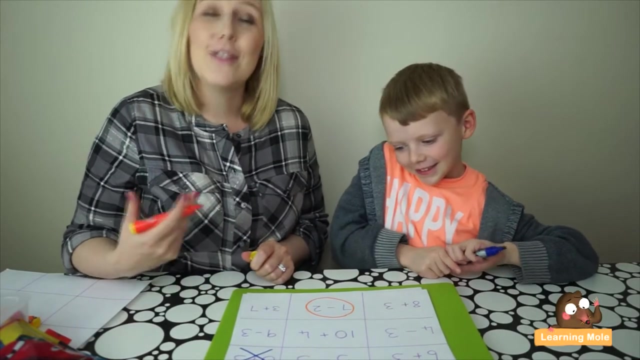 Okay, you ready, Mm-hmm. So now you have to check if I'm correct or not. Mm-hmm Seven, and I've got my two fingers. Six, five. My answer is five, Am I correct? This is a nice opportunity as well to get your child to double check your calculations. 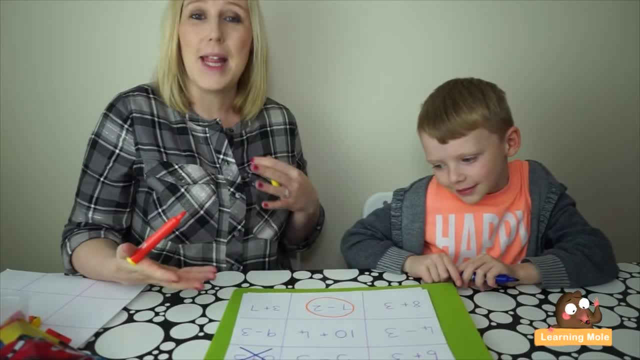 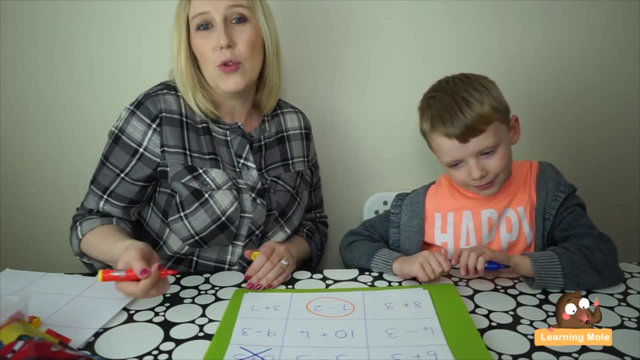 So do feel free to make the odd wee mistake. It shows them that they that making mistakes absolutely fine and it's natural, but also it gives them a chance to really think about what you're doing as well. Okay, next one, Aaron. what are you going to do now? 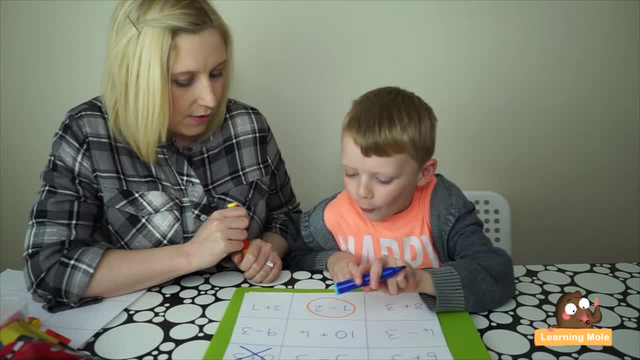 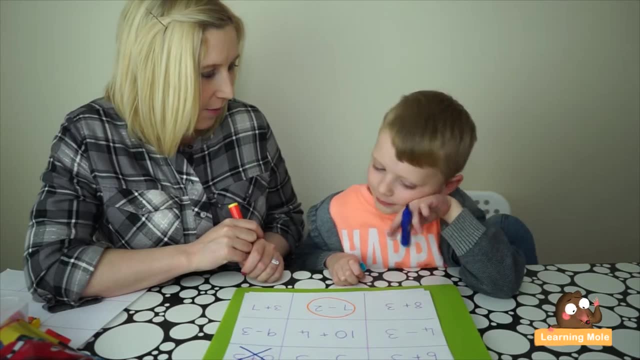 What's that? What's the calculation? say Ten plus four. Oh, can you think of another word? that means the same thing, Same as plus Odd Good boy, right? So tell me what you're going to do. What number are you going to put in your head? 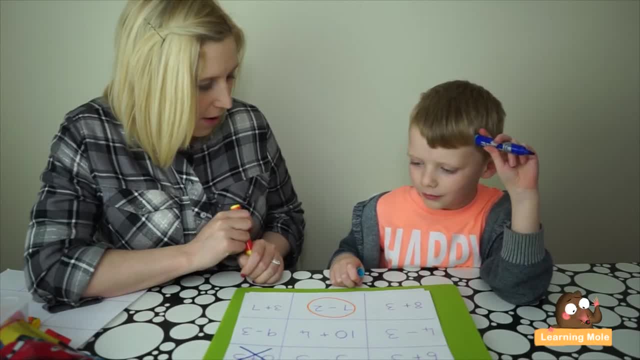 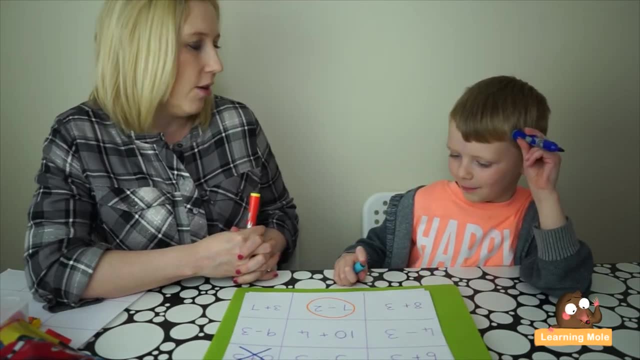 First: Hmm, four. Well, is four the biggest number? No, What do you think? Would it be easier to put ten in your head, because it's the biggest number? Yeah, Yeah, okay. And then what are you going to do? 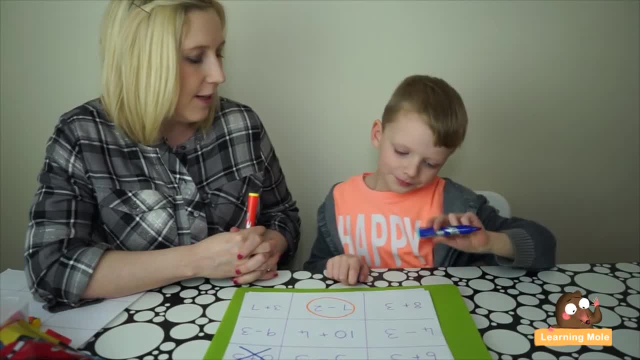 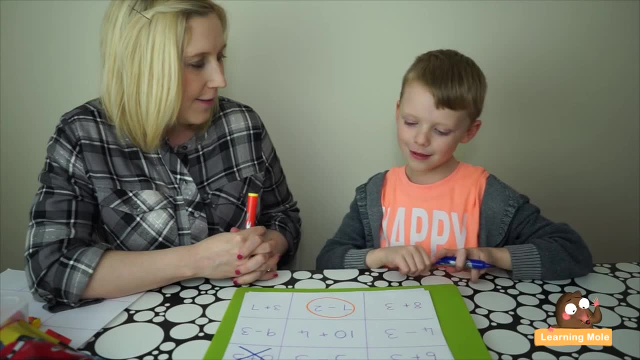 I put four in it. Okay, right, So off you go. My answer is four, Okay, Nine, ten, eleven, twelve, thirteen, fourteen, Right, let me check. Ten, eleven, twelve, thirteen, fourteen, Yes, 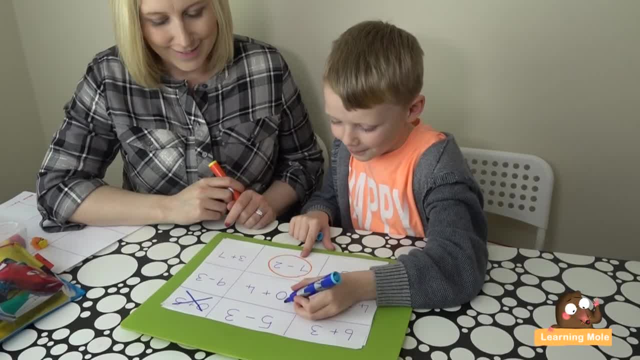 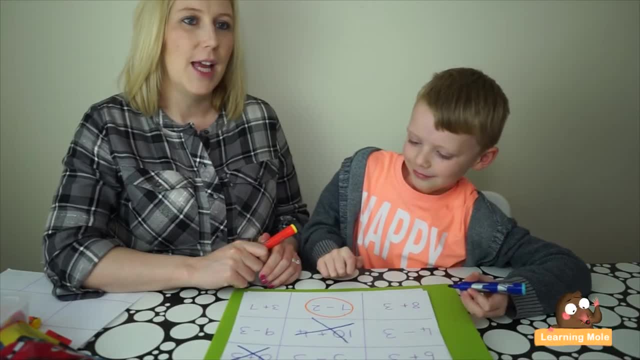 Uh-oh, Oh, I'm going to have to try and block you now. Okay, so I'll have to do eight plus three. Okay, so I'm going to put three in my head first. Do you think that would be a good idea? 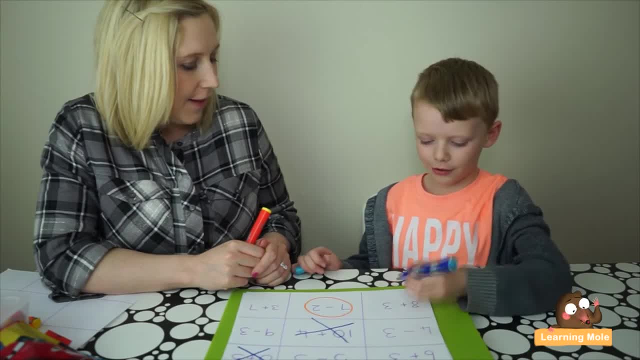 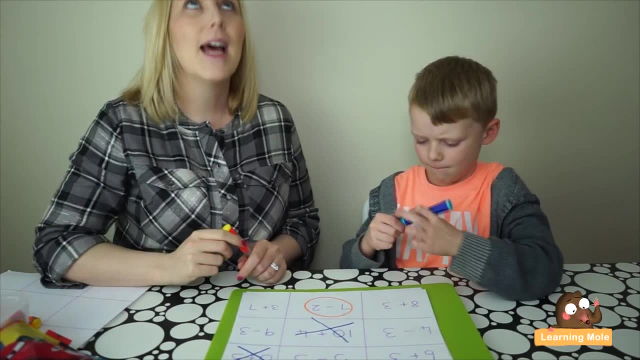 No, Why not? Because you should always put the biggest number. Oh, okay, Okay, so eight You ready? Mm-hmm, Ten eleven, Ten eleven. My answer is eleven, Am I correct? Ooh, I blocked you. 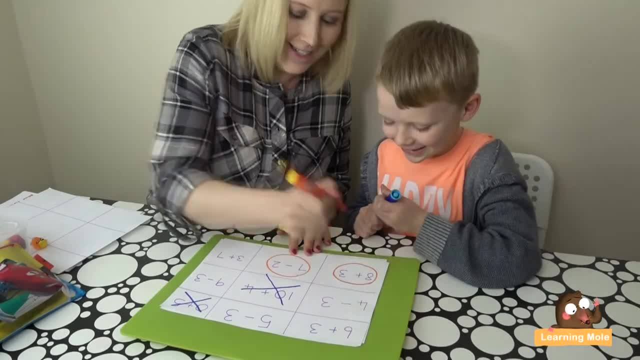 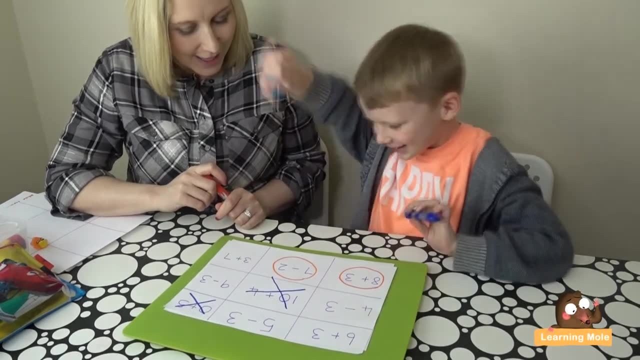 Well, Okay, right now. three plus seven. Three plus seven. okay, I'm going to block you. Oh no, sneaky. Okay, tell me How are you going to do it. First, put seven in your head. 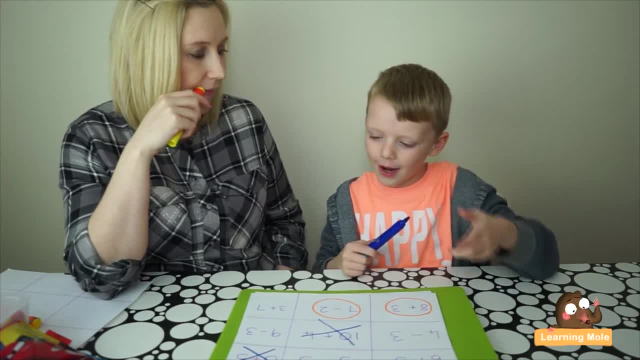 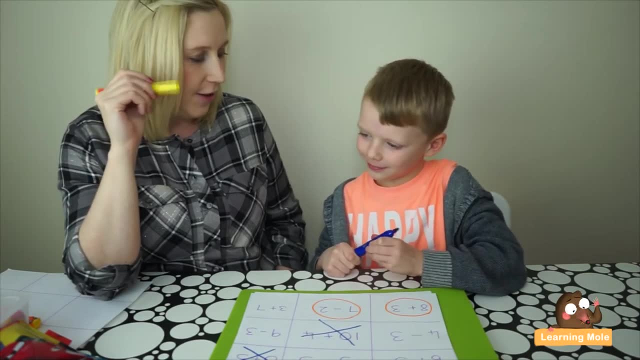 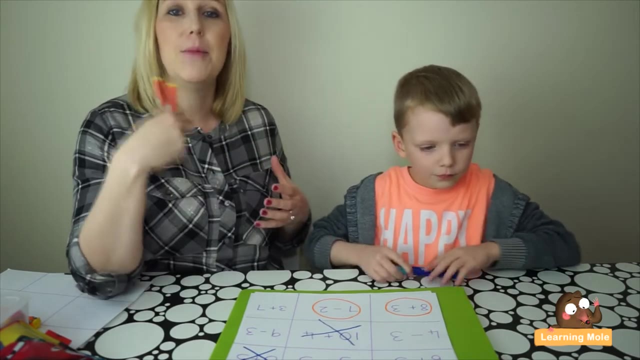 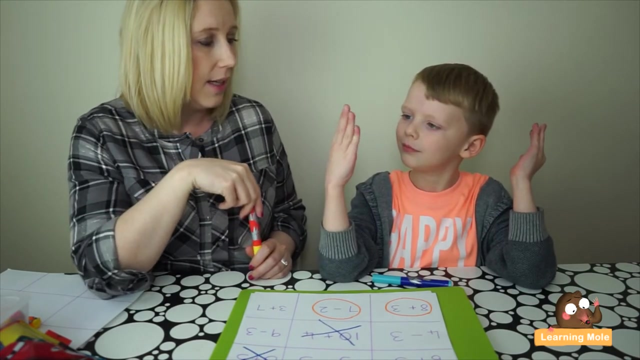 Good, and then you're going to add on Three. Okay, good off you go then. so just keep encouraging your child to reinforce that idea of putting that biggest number in their head first and to reinforce the idea of actually talking through what they are trying to do in their heads, because once they can verbalize it, they know exactly what. 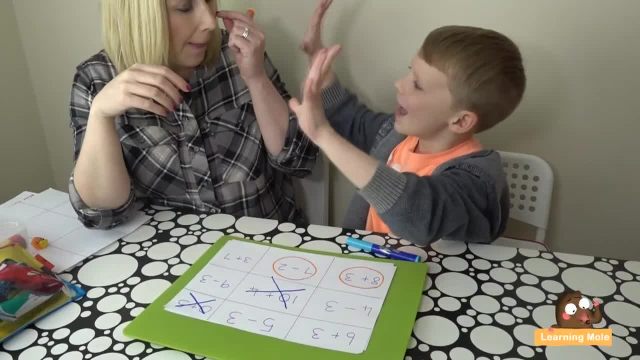 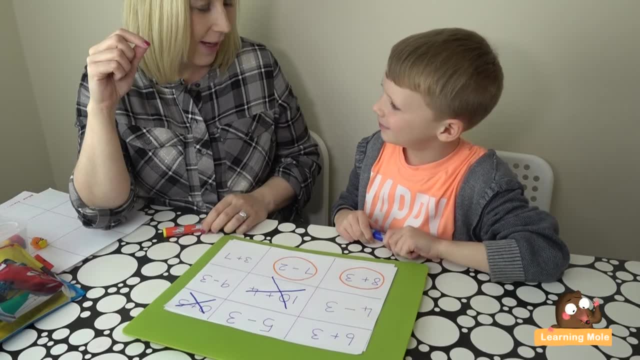 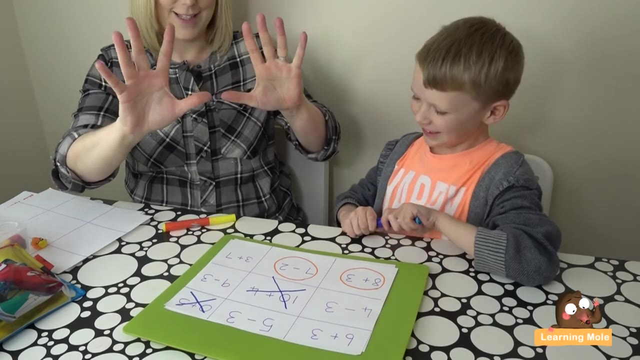 they're doing, and so do you, so you can actually help them. okay, let me check. this time i'm not going to put it in my head, i'm going to put it on my fingers. okay, so i'm going to do seven fingers and then i'm going to add on three, one, two, three, ten. you are correct. 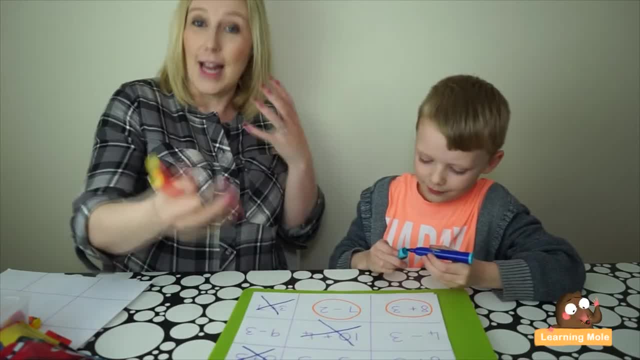 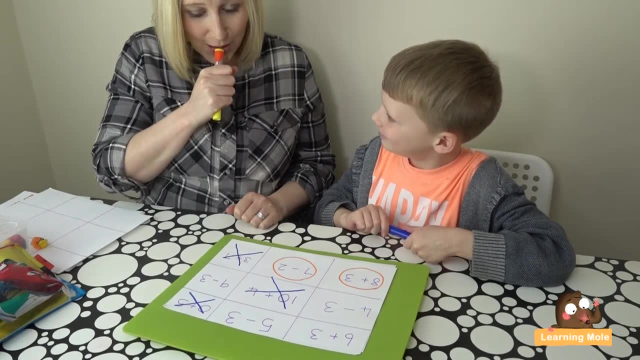 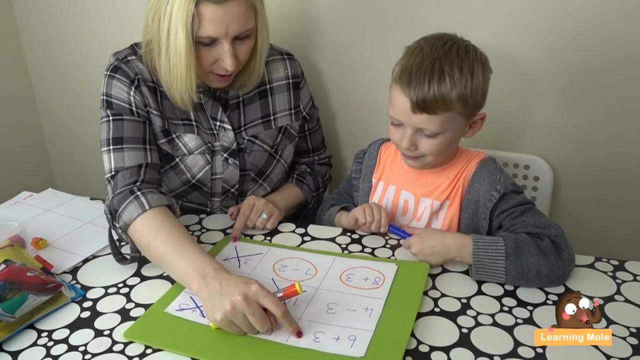 do show your child as well. there are different ways of solving, like using your fingers, or counting forward, or counting backwards as well. oh, oh no, i don't know if i can. if i go there, i can't block you. if i go there, i don't think i can block you. oh, i'll try here, okay. 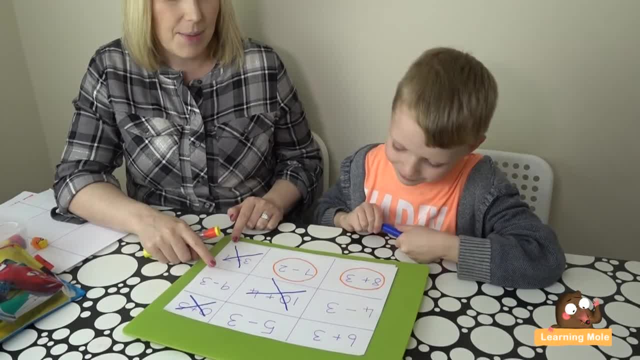 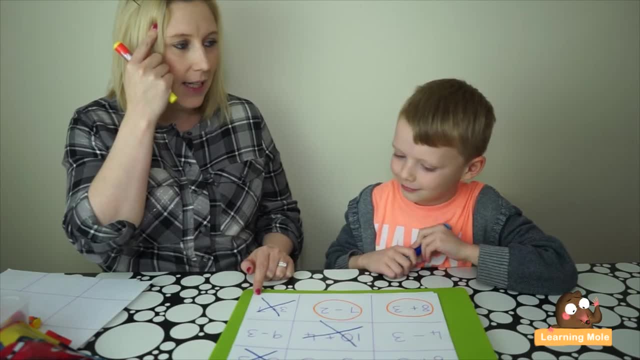 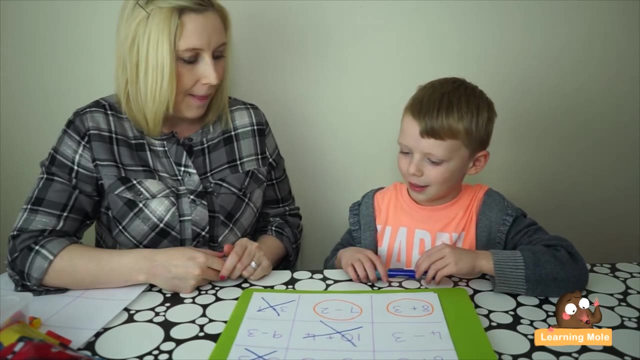 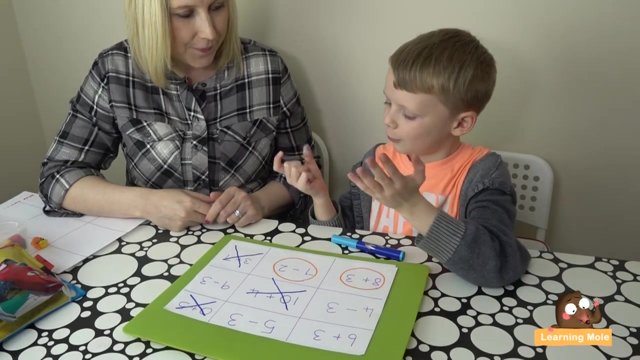 right, nine minus three, okay, so this time i have to count backwards, okay, so are you ready? nine, eight, seven, six, five, am i right? what are you doing wrong? you're wrong, oh no. six, oh no. do you get a chance to solve this number every day in your life? each other's house is all we can have, so don't Distribute it If You Can't Do It Again At Last.